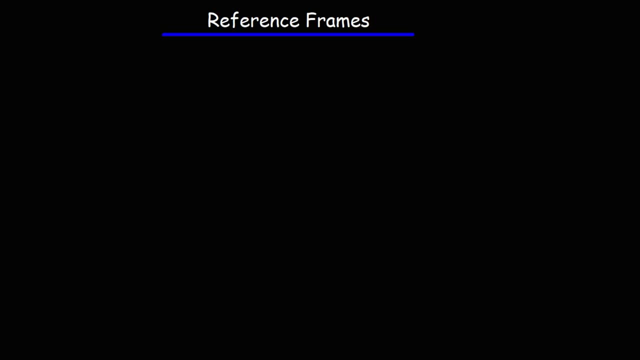 You need to speak about its velocity with respect to something, And that something is the reference frame. For example, you can say that an airplane is moving at 200 meters per second relative to the ground. In this case, the ground would be the reference frame. 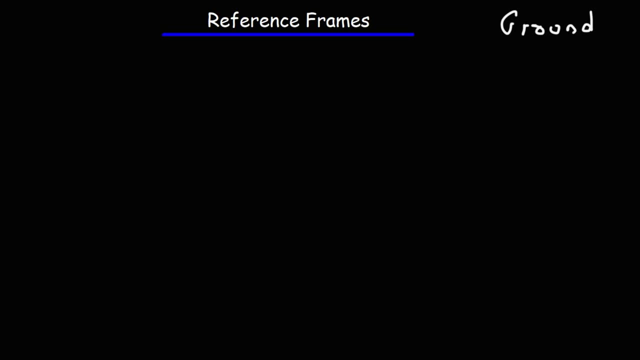 You could say that a car is moving 20 meters per second relative to a bus. In that case, the bus would be the reference frame. What that means is that the car is moving faster than the bus, but you don't really know the car speed relative to the ground. 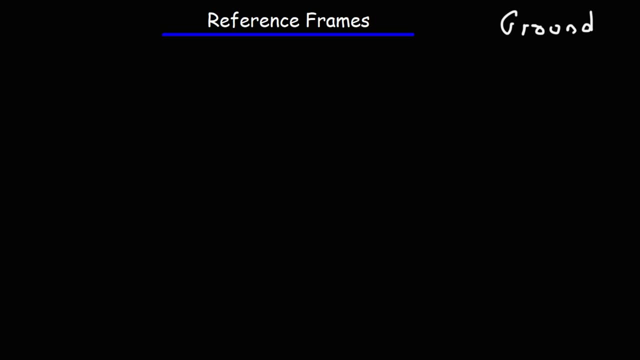 So whenever you're talking about an object's motion, you need to compare it with something, and that something is the reference frame. So let's look at some examples. Let's say we have a person. We'll call this person John. John is moving at a speed of 2 meters per second to the right. 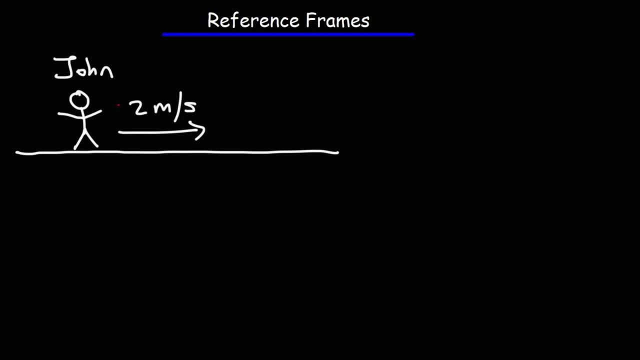 So his velocity is positive too. Now, what's the reference frame? in this example, If the reference frame is not specified, it's typically assumed to be the ground. In this case it is. John is moving 2 meters per second relative to the ground. 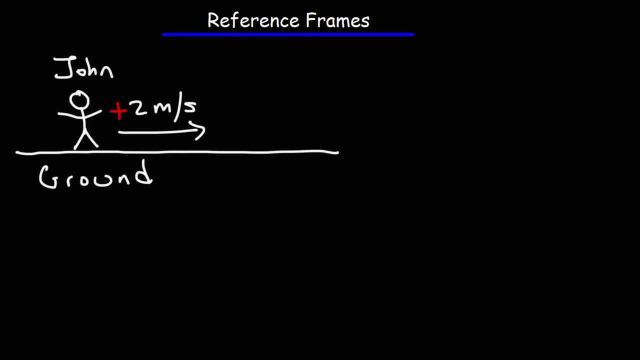 So the ground is the reference frame. Now I'm going to change the units of his velocity, because to move at a speed of 2 meters per second, that's actually quite fast for a person. So let's say it's 2 miles per hour. 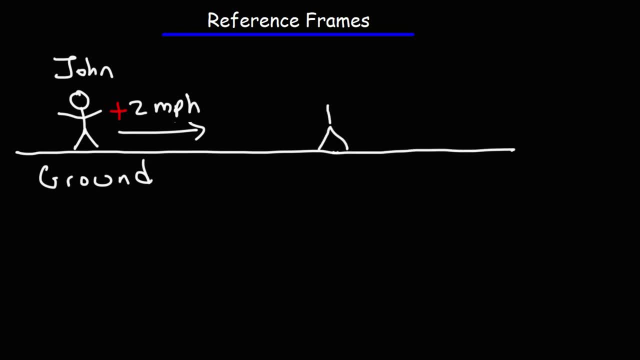 Now we're going to have another person. We'll call this person Sally, And let's say that Sally is moving at a velocity of 3 miles per hour towards the right, And that's relative to the ground. So we'll call this VJG. 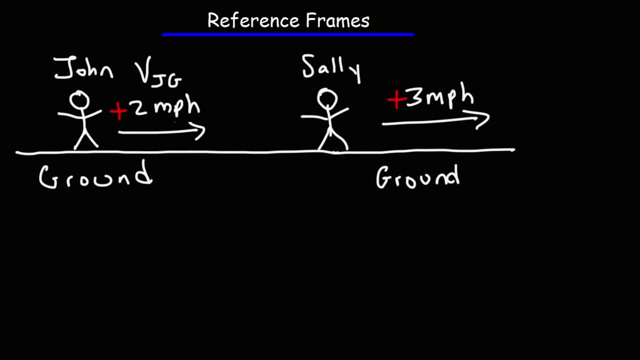 That is John's velocity relative to the ground, And we'll call this VSG- Sally's velocity with respect to the ground. Now here's a question for you: What would be the value of VSJ? What is Sally's velocity relative to John? 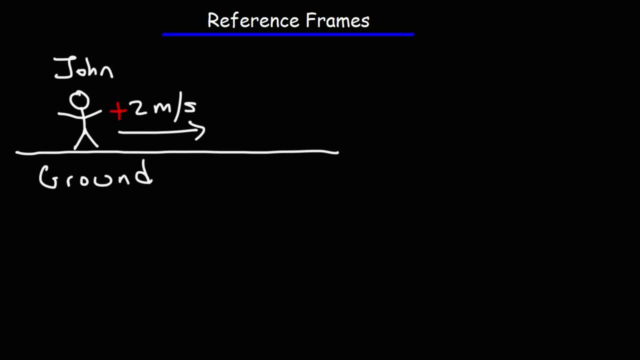 per second relative to the ground. so the ground is the reference frame. now I'm going to change the units of his velocity, because to move at a speed of two meters per second, that's actually quite fast for a person. so let's say it's two miles per hour. now we're gonna have another person. we'll call this person. 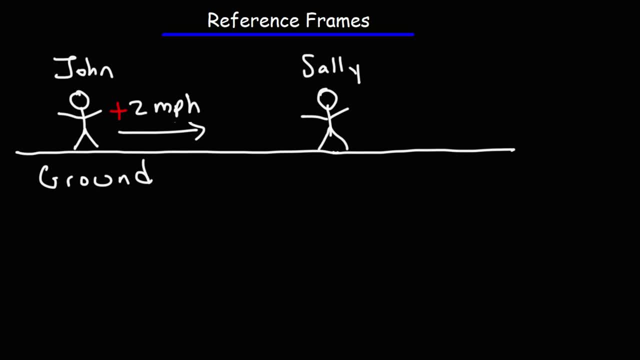 Sally, and let's say that Sally is moving at a velocity of three miles per hour towards the right, and that's relative to the ground- ground. So we'll call this VJG. That is, John's velocity relative to the ground, And we'll call 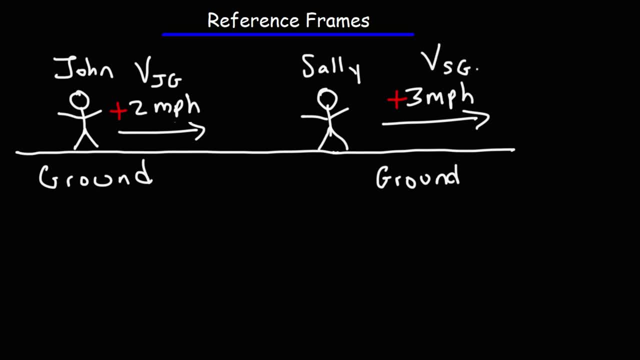 this VSG, Sally's velocity with respect to the ground. Now here's a question for you: What would be the value of VSJ? What is Sally's velocity relative to John? Well, Sally is moving faster than John. From John's perspective. every hour Sally is going to be one mile ahead of him. 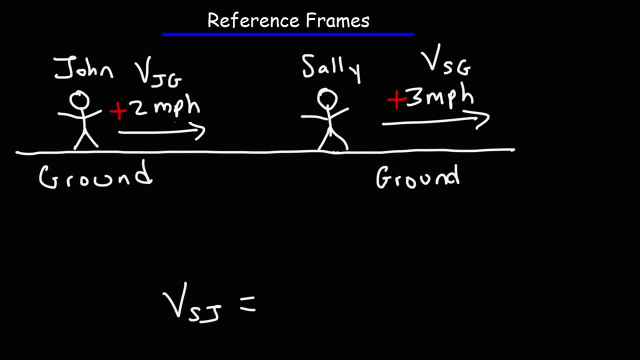 She's moving one mile per hour faster than he is, So the distance between John and Sally will continue to increase. From John's perspective, Sally is moving away from him. So, Sally, her speed is one mile per hour greater than John. Now we can also say what is John's velocity relative to Sally. 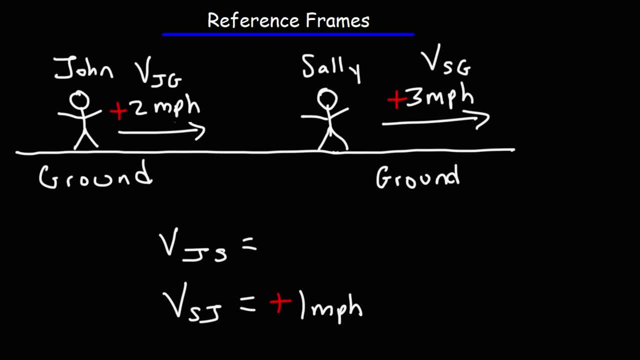 Well, John is moving slower than Sally. From Sally's perspective it appears as if John is moving away from her because she's moving ahead of him. So his velocity relative to her is actually going to be negative one miles per hour. So in this case, for this value, the reference frame is John, because we're looking at Sally's. 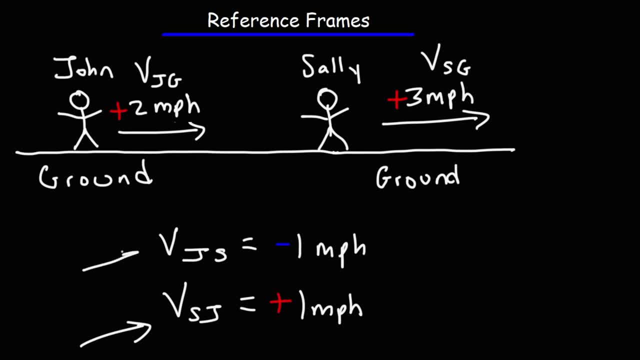 velocity relative to John, And for this value, the reference frame is Sally, because we're looking at John's velocity with respect to Sally's. Now, for those of you who like to have formulas, here's how you can get the answer using a formula. 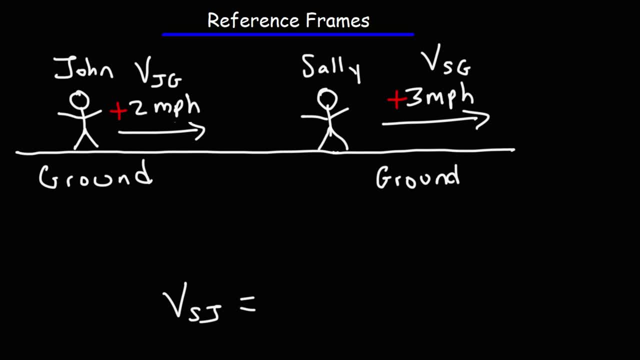 Well, Sally is moving faster than John than John. from John's perspective. every hour, Sally is gonna be one mile ahead of him. she's moving one mile per hour faster than he is, so the distance between John and Sally will continue to increase. from John's perspective, Sally- 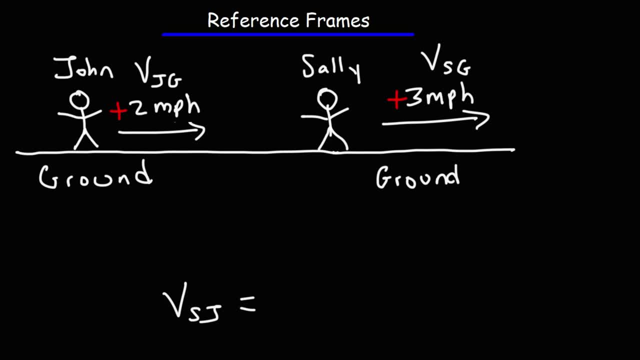 is moving away from him, so Sally, her speed is one mile per hour and greater than John. now we can also say what is John's velocity relative to Sally? well, John is moving slower than Sally. from Sally's perspective, it appears as if John is moving away from her because she's moving ahead of him, so his 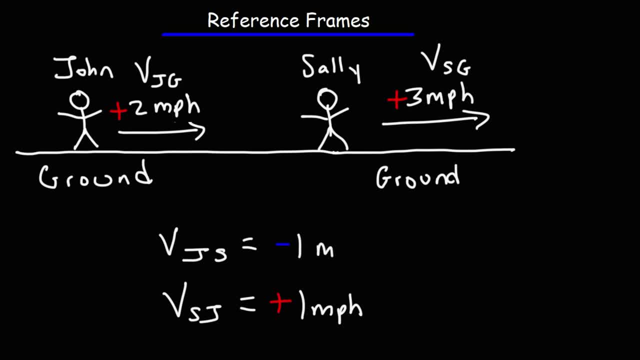 velocity relative to her is actually gonna be negative: 1 miles per hour. so in this case, for this value the reference frame is John, because we're looking at Sally's velocity relative to John, and for this value the reference frame is Sally because we're looking at John's velocity with respect to Sally's. now for those of you who like, 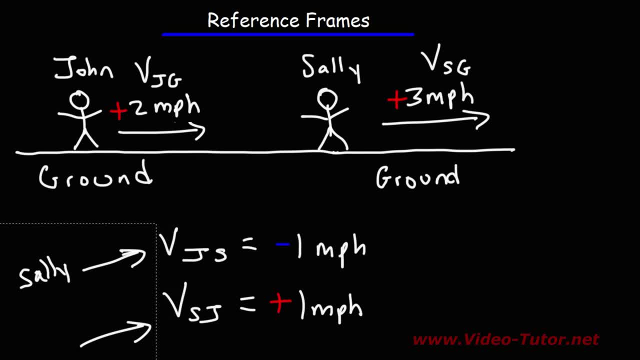 to have formulas. here's how you can get the answer. using the formula, the velocity of John relative to Sally is going to be negative 1 miles per hour, so the reference frame is 3 miles per hour. so this is our reference frame for the velocity of John and Sally. it's basically the difference between the two. it's 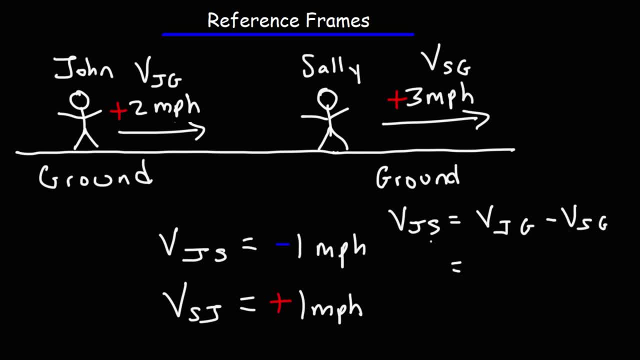 John's velocity relative to the ground minus Sally's velocity relative to the ground. so V J s is going to be V J minus V s, but both with respect to the ground. and it makes sense if we plug in the numbers 2 minus positive 3 will give 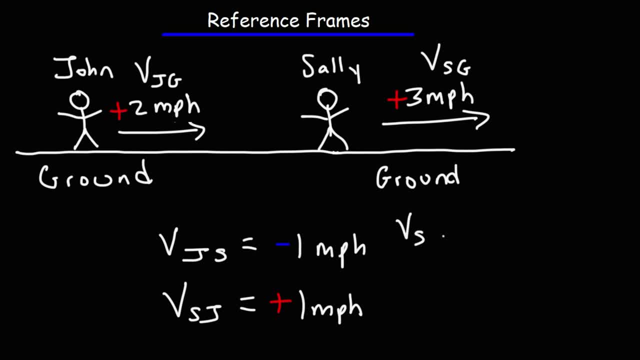 us negative 1. Sally's velocity relative to John is going to be Vs minus Vj, but Sally's velocity relative to the ground minus John's velocity relative to the ground. So Vsj is 3 minus Vjg, which is positive 2, and that gives us positive 1.. So 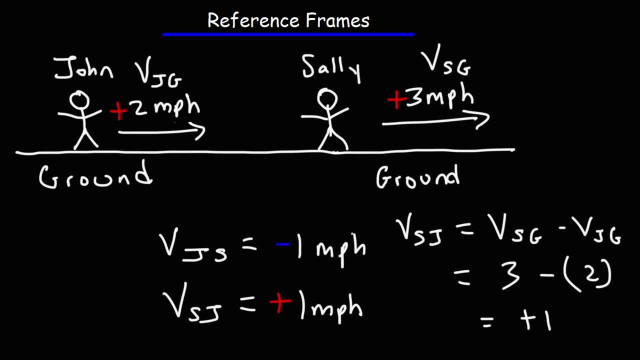 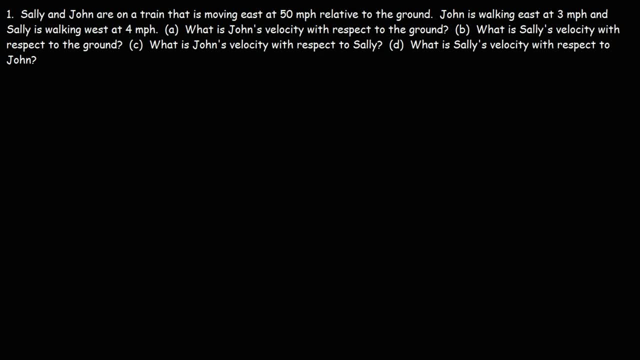 that's the math behind the operations that gave us these two answers. Now let's work on an example problem. Sally and John are on a train that is moving east at 50 miles per hour. relative to the ground, John is walking east at 3 miles. 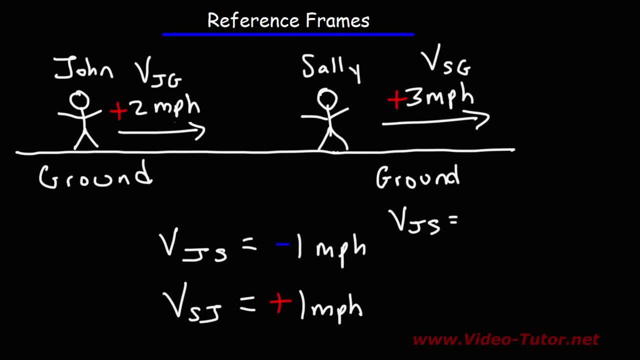 The velocity of John relative to Sally is basically the difference between the two. It's John's velocity relative to the ground minus Sally's velocity relative to the ground. So vjs is going to be vj minus vs, but both with respect to the ground. 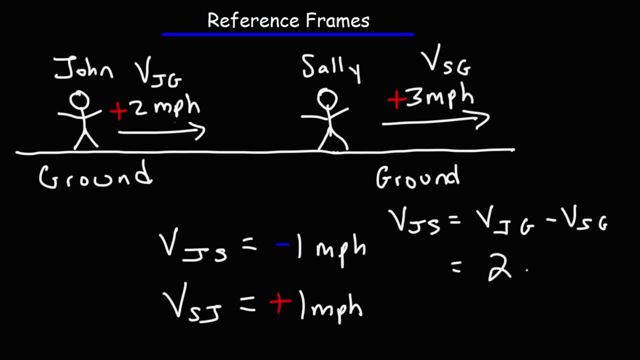 And it makes sense. If we plug in the numbers 2 minus positive 3 will give us negative 1.. Likewise, to calculate Sally's velocity relative to John, it's going to be Vs minus Vj, But Sally's velocity relative to the ground minus John's velocity relative to the ground. 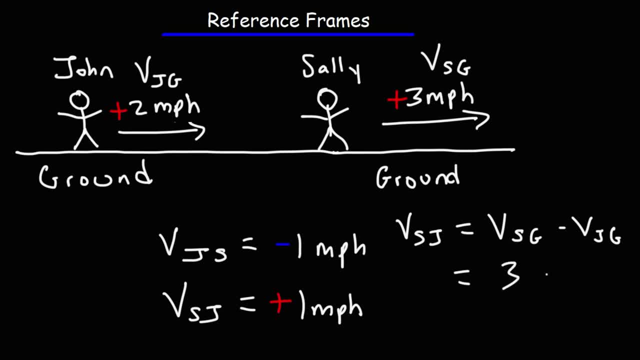 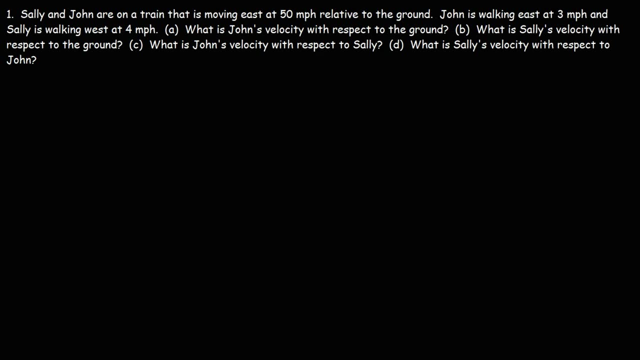 So Vsj is 3 minus Vjg, which is positive 2, and that gives us positive 1.. So that's the math behind the operations that gave us these two answers. Now let's work on an example problem. Sally and John are on a train that is moving east at 50 miles per hour relative to the ground. 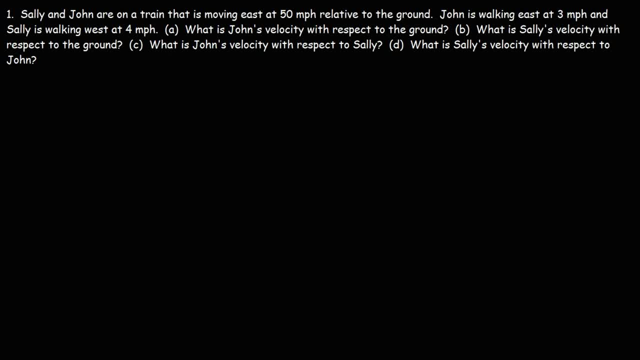 John is walking east at 3 miles per hour And Sally is walking west at 4 miles per hour. What is John's velocity with respect to the ground? So let's draw a picture. So that's going to be the ground, And let's draw a picture of a train. 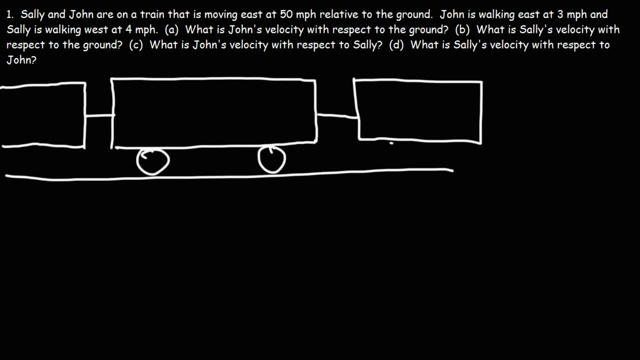 Now on this train, we see that John is walking east at 3 meters per second. What's the velocity in this? What's the position of these bystanders? What's the color of the sky around them? What's the part of the sky around them? What's the constant time it takes for them to move west? Does any crossing depend on the distance? What's the position of theEsq far from Darnell high street という? many years ago, we used to say that John needed a greater, greater velocity than us. So what would beatta says, is this Ready or Not? while also asking: what did thehmтуatsart have to do? I wouldn't say that I would have to say any of them today. One thing that we just said was that we need to write out there those things when we note down these results. 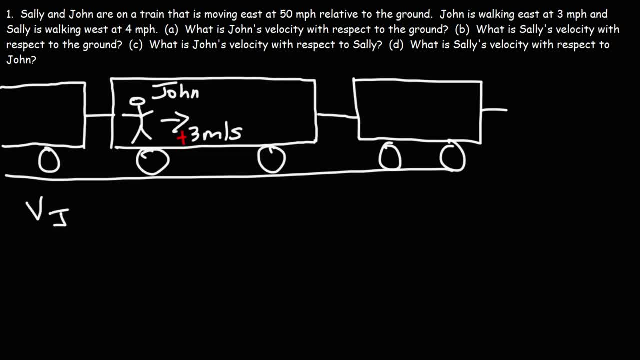 So these aren't Bharath, let me say this. So we could say that John's velocity relative to the train is positive 3 meters per second, or rather miles per hour. Let's fix that. But what is his velocity relative to the ground? 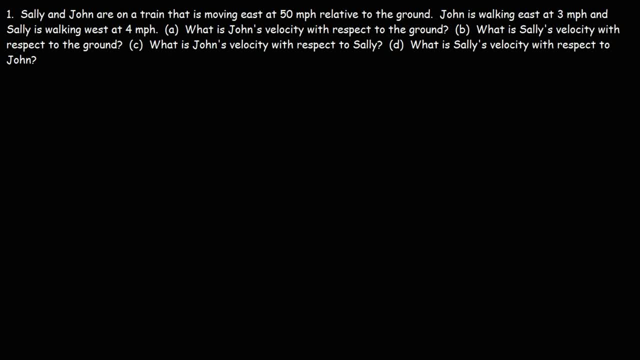 per hour and Sally is walking west at 4 miles per hour. What is John's velocity with respect to the ground? So let's draw a picture, So that's gonna be the ground, and let's draw a picture of a train. Now, on this train. 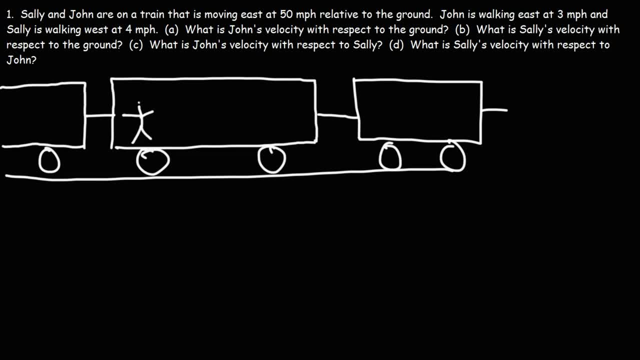 we see that John John is walking east at 3 meters per second. So we could say that John's velocity relative to the train is positive: 3 meters per second, or rather miles per hour. Let's fix that. But what is his velocity? 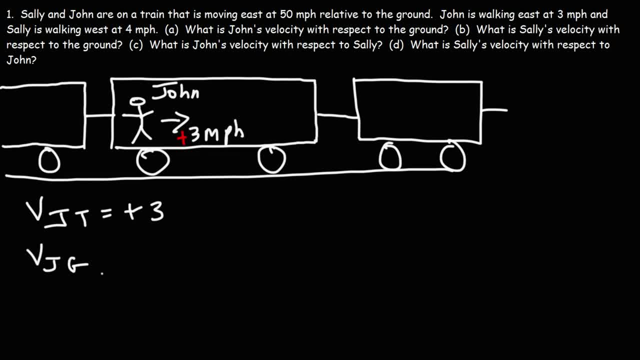 relative to the ground. So an observer who is standing on the ground, what does he see? An observer standing from the ground, he sees the train moving at 50 miles per hour to the right, relative to him. Now, in addition to that, 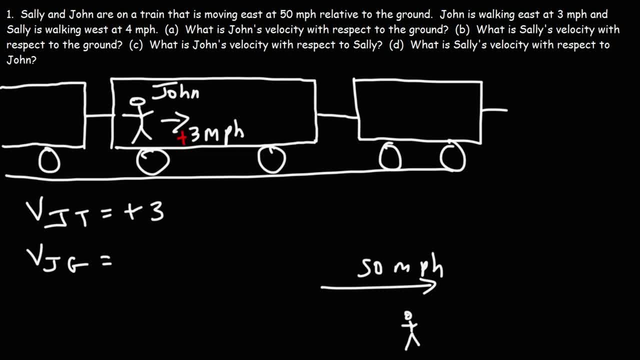 John is walking to the right. He's walking 3 miles per hour faster than the train, So John's velocity is positive 3 meters per second. So John's velocity relative to the train, with respect to the ground, as viewed by an observer, is actually going to be. 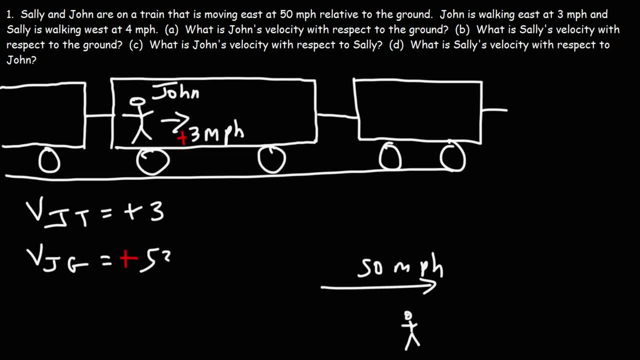 positive 53 miles per hour. It's going to be the sum of the train and the velocity, because they're both moving in the same direction. Now, for those of you who like to use a formula to see the calculations, here's what you can do. 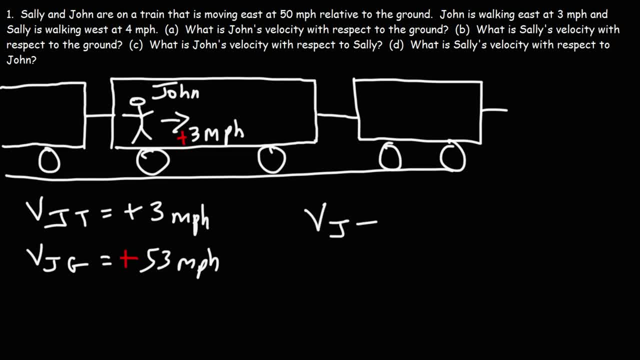 So John's velocity with respect to the train is going to be, or in other words, VJT is going to be, VJ with respect to the ground minus VT with respect to the ground. So VJT- John's velocity with respect to the train. 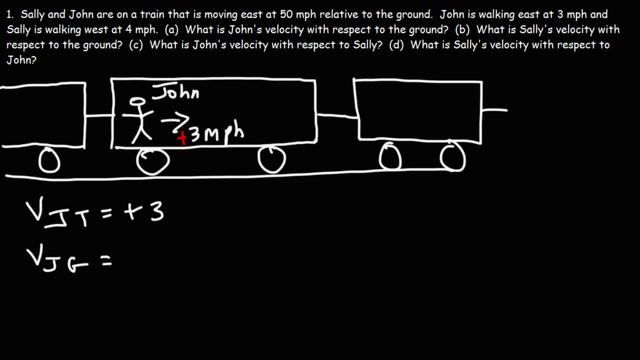 So an observer who is standing on the ground. what does he see? An observer standing from the ground. he sees the train moving at 50 miles per hour to the right relative to him. Now, in addition to that, John is walking to the right. 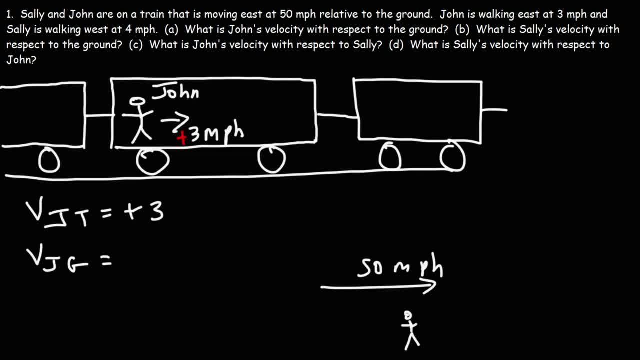 He's walking 3 miles per hour faster than the train. So John's velocity With respect to the ground, as viewed by an observer, is actually going to be positive 53 miles per hour. It's going to be the sum of the train and the velocity, because they're both moving in the same direction. 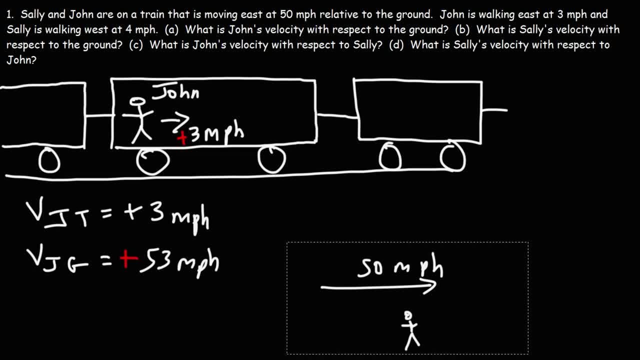 Now for those of you who like to use a formula to see the calculations, here's what you can do: John's velocity, John's velocity, John's velocity with respect to the train is going to be, or in other words, VJT is going to be VJ with respect to the ground, minus VT with respect to the ground. 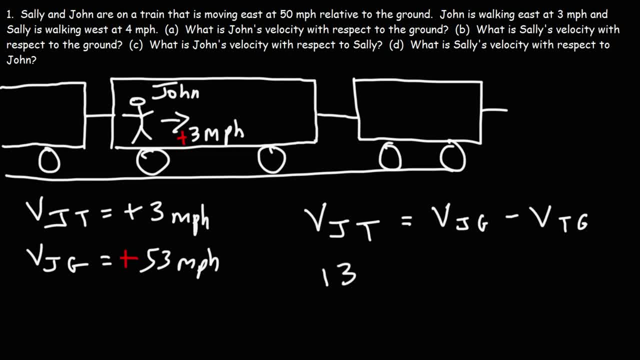 So VJT, John's velocity with respect to the train, that's positive 3.. We're looking for John's velocity with respect to the ground And the train's velocity with respect to the ground. we know it's positive 50.. 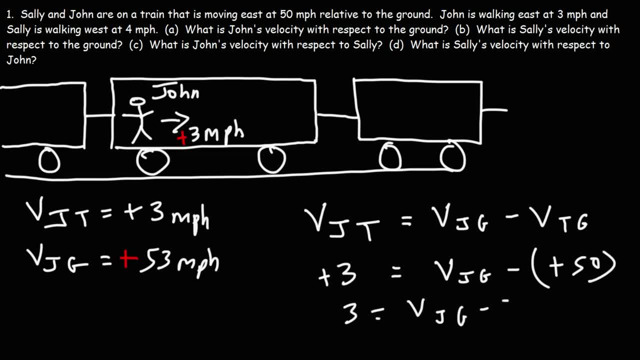 So what we have is 3 equals VJT, VJT minus 50. Well, to get this answer, we need to add 50 to both sides. So, moving negative 50 to the other side, it's going to be positive 50 minus. I mean plus 3.. 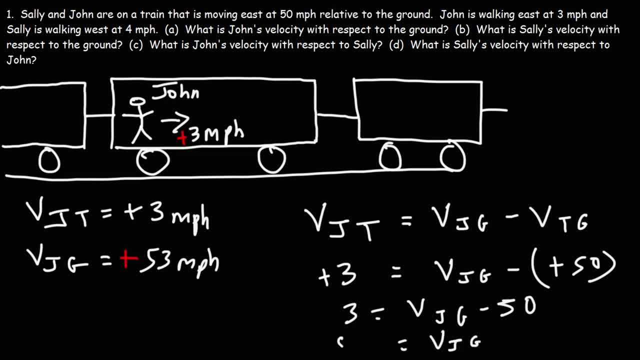 And that's how we get VJT is positive 53. So that's how you can use the formula to get that answer. Now let's move on to part B. What is Sally's velocity with respect to the ground? So Sally, 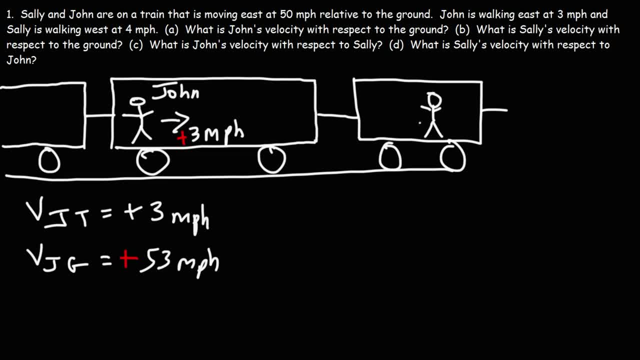 Sally is moving west at 4 miles per hour, and this is while she's on the train. So Sally's velocity with respect to the train is negative 4 miles per hour. It's negative because she's moving to the left. Now what is her velocity with respect to the ground? 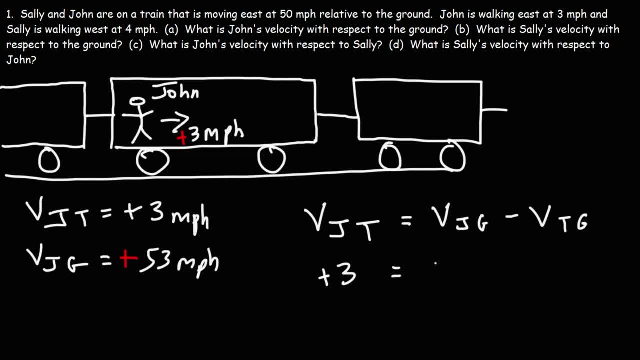 that's positive 3.. We're looking for John's velocity with respect to the ground and the train's velocity with respect to the ground. we know it's positive 50.. So what we have is 3 equals VJG minus 50.. 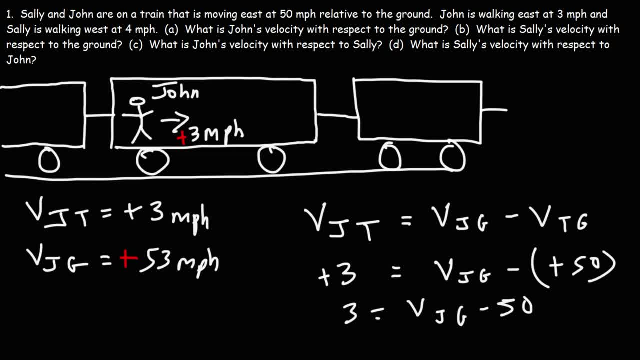 Well, to get this answer, we need to add 50 to both sides. So, moving negative 50 to the other side, it's going to be positive 50 minus, I mean plus 3. And that's how we get VJG is positive 53.. 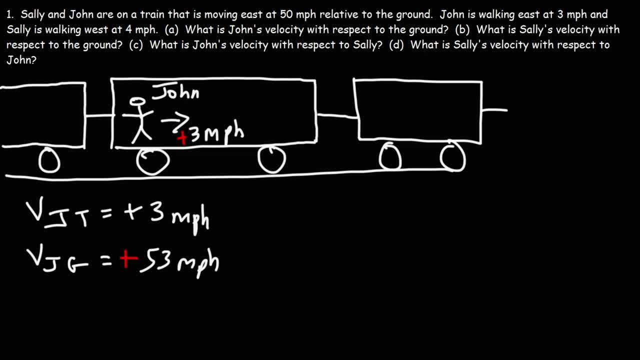 So that's how you can use the formula to get that answer. Now let's move on to part B. What is Sally's velocity with respect to the ground? So Sally is moving west at 4 miles per hour, and this is while she's on the train. 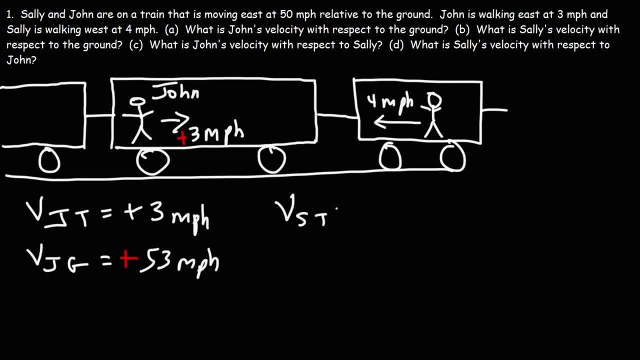 So Sally's velocity with respect to the train is negative: 4 miles per hour. It's negative because she's moving to the left. Now what is her velocity with respect to the ground? Well, we could use the same formula or something similar to it. 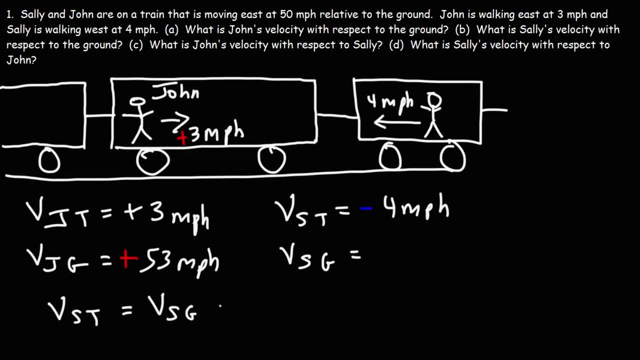 So VST is going to be VS with respect to the ground minus VT with respect to the ground. VST is negative 4.. VSG is what we're looking for And the velocity of the train with respect to the ground is negative 50.. 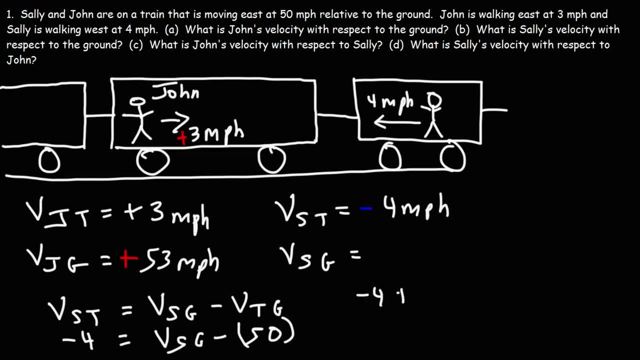 So we need to add 50 to both sides. So it's going to be negative 4 plus 50 and that's going to equal VSG Negative 4 plus 50, that's going to be positive 46.. So to an observer on the ground, 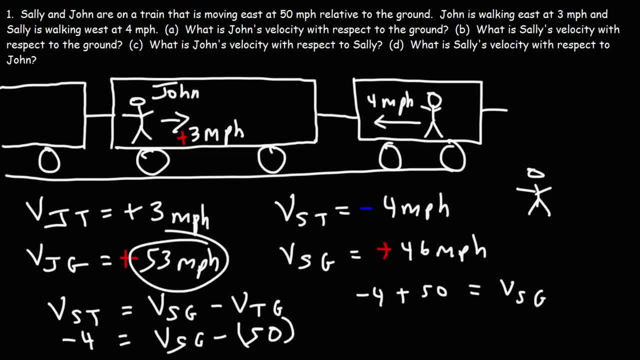 John is moving east. So John will appear to be moving faster than the ground, than the train. Sally's moving west. So to an observer on the ground, Sally is going to be moving slower than the train. She's still moving to the right. 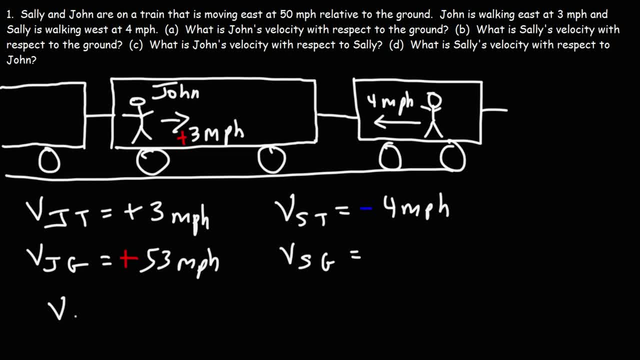 Well, we could use the same formula or something similar to it. So VST is going to be VS with respect to the ground, minus VT. with respect to the ground, VST is negative 4.. VSG is what we're looking for. 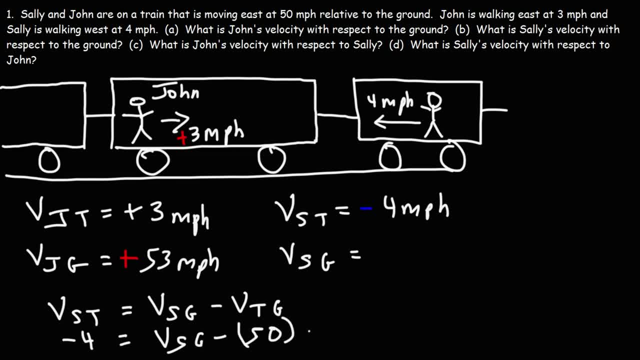 And the velocity of the train with respect to the ground is negative 50. So we need to add 50 to both sides. So it's going to be negative 4 plus 50, and that's going to equal VSG. 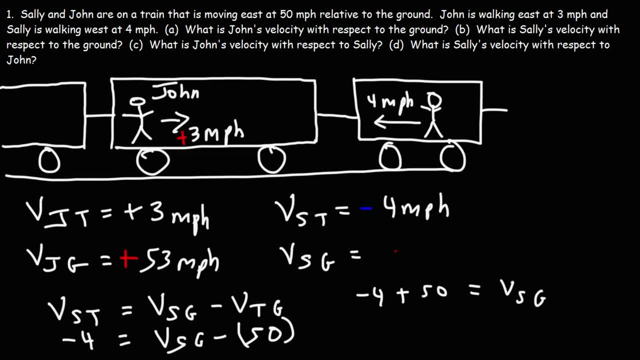 Negative 4 plus 50, that's going to be positive 46. So, to an observer on the ground, John is moving east. So John will appear to be moving faster than the train. Sally's moving west. So, to an observer on the ground, Sally is going to be moving slower than the train. 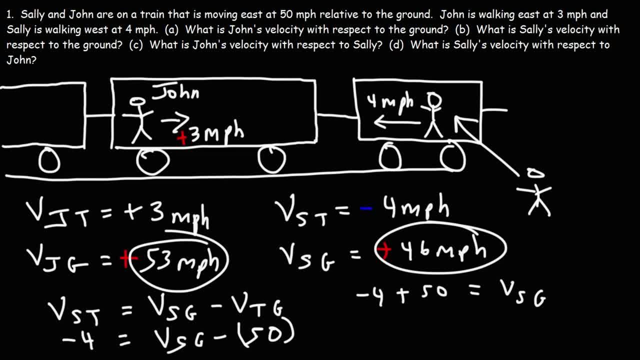 She's still moving to the right with respect to the observer, but she's moving at a slower rate relative to the train. Now let's move on to Part C. What is John's velocity with respect to Sally? So we're looking for VJF. 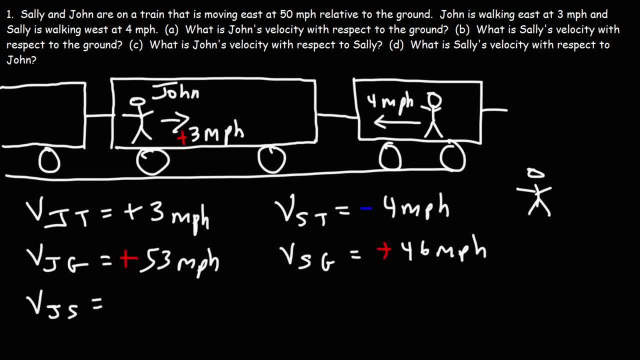 That's John's velocity with respect to Sally. Using the formula, it's going to be John's velocity with respect to the ground minus Sally's velocity with respect to the ground, And we have those numbers. It's those two numbers, So it's going to be 53 minus positive 46.. 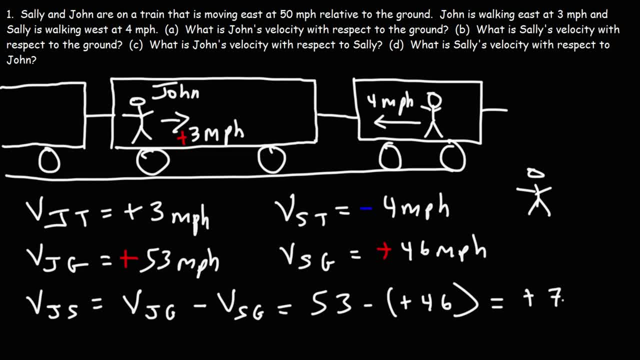 53 minus 46, that's positive 7. So John's velocity relative to Sally is positive 7. What that means is that his velocity is 7 units greater than Sally's velocity, Which makes sense. Positive 3 is 7 more units than negative 4.. 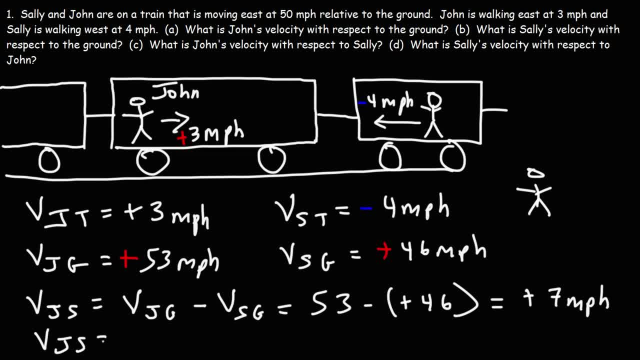 Now we can also get the same answer using this formula. Instead of using the ground as the common reference frame, we can use the train as a common reference frame, Because both of them are the same. Both John and Sally are on the train. 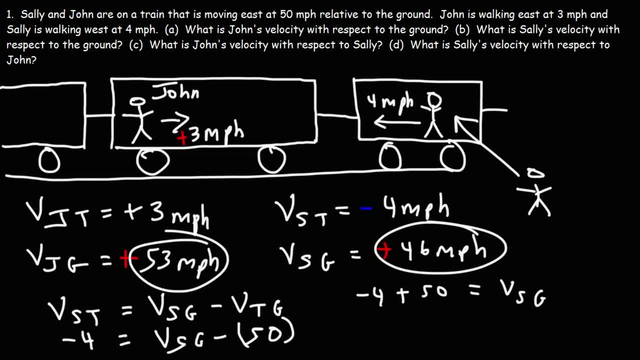 with respect to the observer, but she's moving at a slower rate relative to the train. Now let's move on to Part C. What is John's velocity with respect to Sally? So we're looking for VJS. John's velocity with respect to Sally. 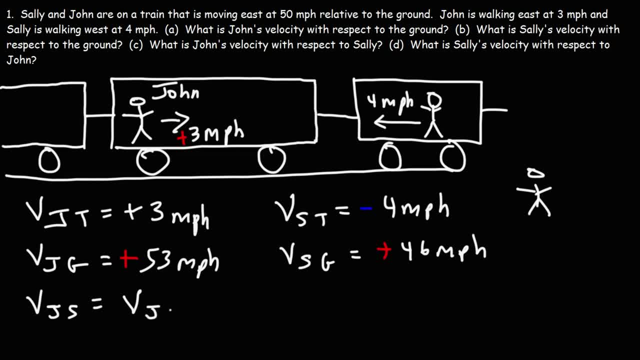 Using the formula, it's going to be John's velocity with respect to the ground minus Sally's velocity with respect to the ground, And we have those numbers. It's those two numbers. So it's going to be 53 minus positive 46.. 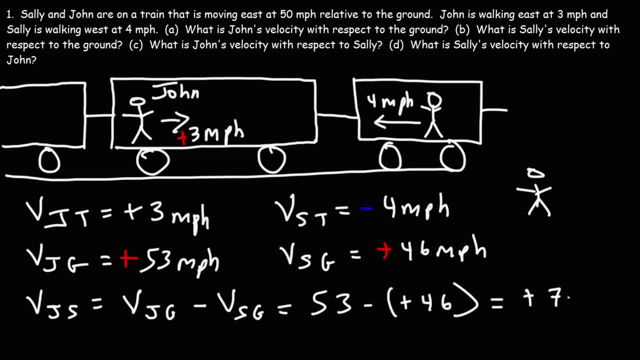 53 minus 46, that's positive 7. So John's velocity relative to Sally is positive 7. What that means is that his velocity is 7 units greater than Sally's velocity, which makes sense. Positive 3 is 7 more units. 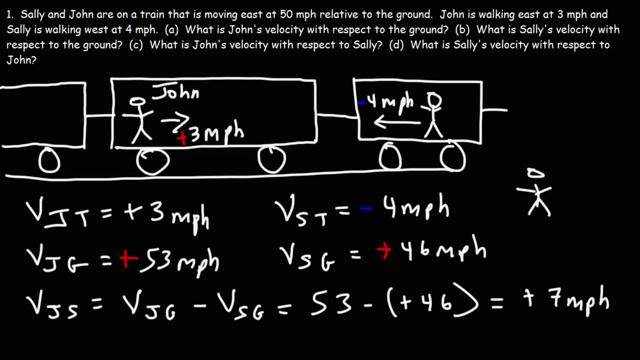 than negative 4.. Now we can also get the same answer using this formula. Instead of using the ground as the common reference, we can use the train as a common reference frame, because both John and Sally are on a train, So VJS can also be calculated. 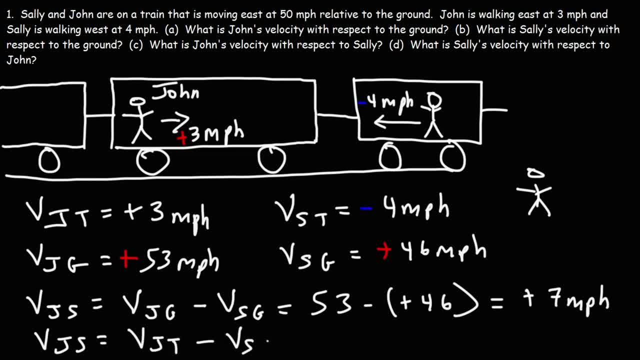 using this formula: VJT minus VST. It works the same as long as we use a common reference frame. So VJT, that's positive, 3, minus VST, which is negative, 4.. 3 minus negative 4 is the same as 3 plus 4.. 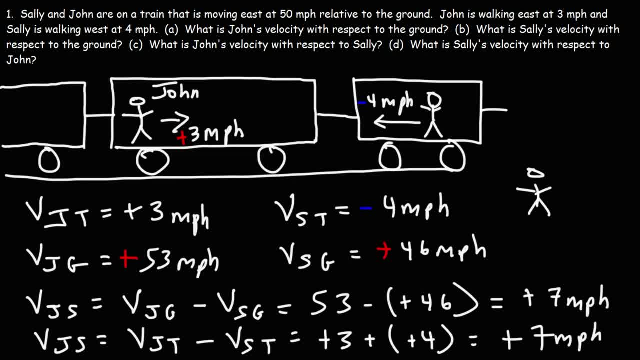 And it gives us positive 7 miles per hour. So that is John's velocity with respect to Sally. Now, what is Sally's velocity with respect to John? All you got to do is switch to sine. So VJS is going to equal negative VSJ. 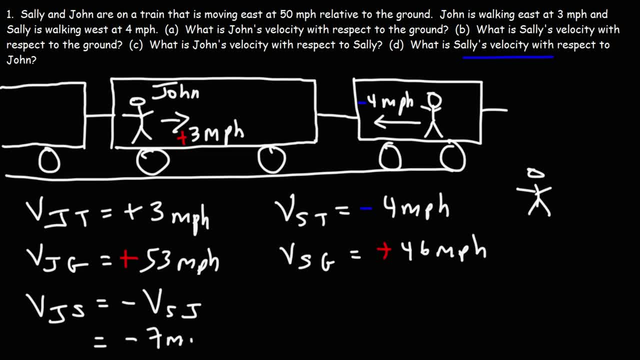 So that means it's going to be negative 7 miles per hour And of course, we can use the formula: VJS is going to be, I mean VSJ, It's going to be VS with respect to the ground, minus VJ. 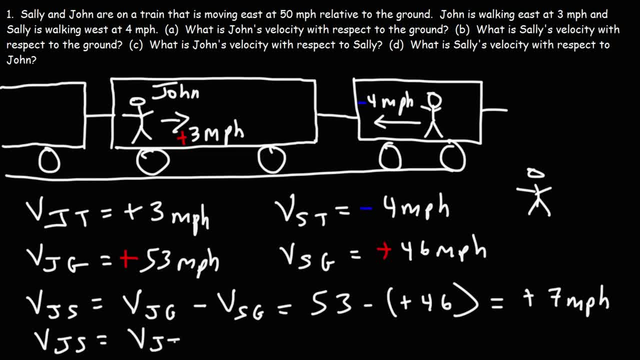 So VJS can also be calculated using this formula: VJT minus VST. It works the same, as long as we use a common reference frame. So VJT, that's positive 3, minus VST, which is negative 4.. 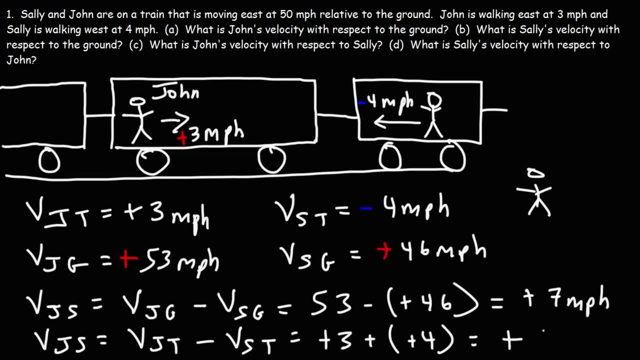 3 minus negative 4 is the same as 3 plus 4. And it gives us positive 7 miles per hour. So that is John's velocity with respect to Sally. Now, what is Sally's velocity with respect to John? 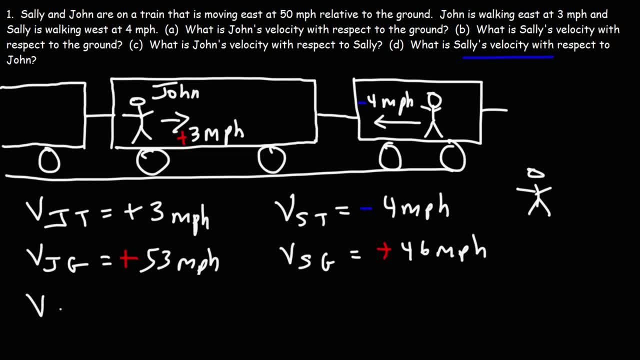 All you got to do is switch to sine. So VJS is going to equal negative VSJ. So that means it's going to be negative 7 miles per hour And of course, we can use the formula VJS is going to be, I mean, VSJ. 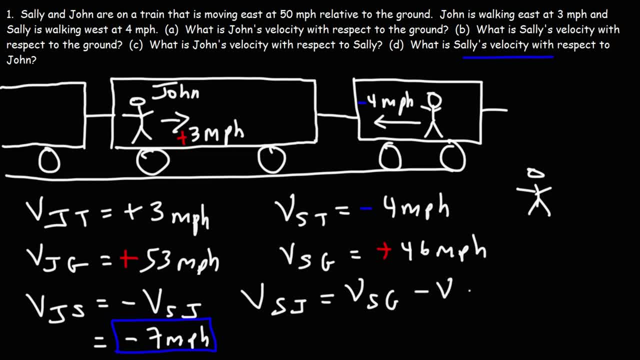 It's going to be VS with respect to the ground minus VJ with respect to the ground, So VSG is 46 minus VJG, which is 53. And that will give us negative 7 miles per hour. So that's Sally's velocity with respect to John. 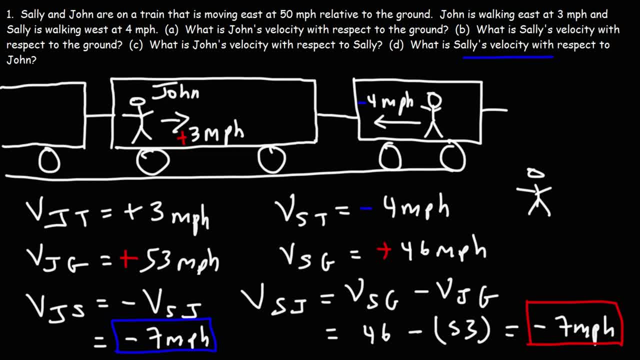 And that's basically it for this video. Hopefully it gave you a good idea into the concept of reference frames. So whenever you describe an object's motion, its velocity, you need to describe it with respect to something, And that something is the reference frame.